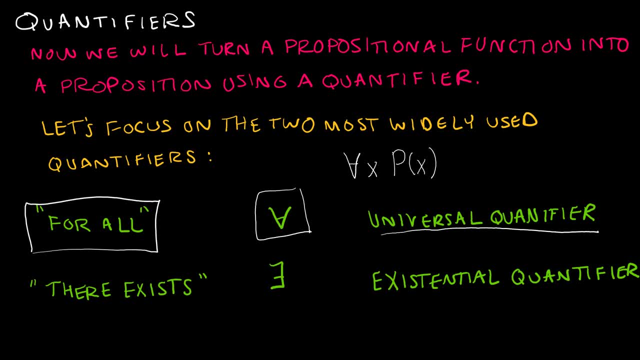 p of x. that would mean for every x. p of x is true, And we're going to talk about both of these in detail on the following slides. The other is the existential quantifier, And that just means there exists, So it's the backwards e, And we're saying there exists some x, So there exists some x. such that p of x is true, And we're going to talk about both of these in detail on the following slides. So there exists some x such that p of x is true, And we're going to talk about both of these in detail on the following slides. So there exists some x such that p of x is true, And we're going to talk about both of these in detail on the following slides. So there exists some x such that p of x is true, And we're going to talk about both of these in detail on the following slides. 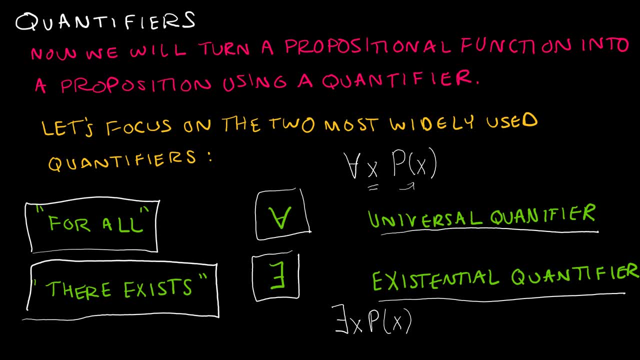 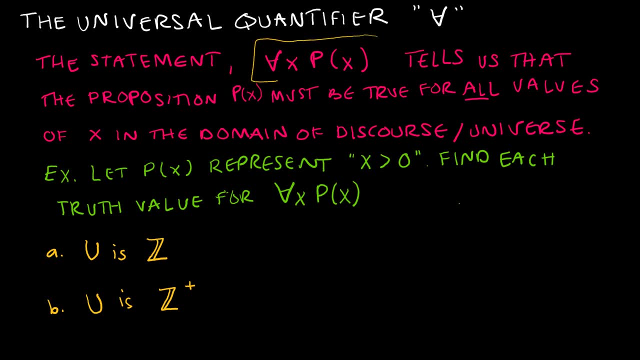 So let's talk a bit more about the universal quantifier. If we have a statement for all x, p of x, that tells us that the proposition p of x must be true for all values of x in the domain of discourse or in the universe, or just domain, 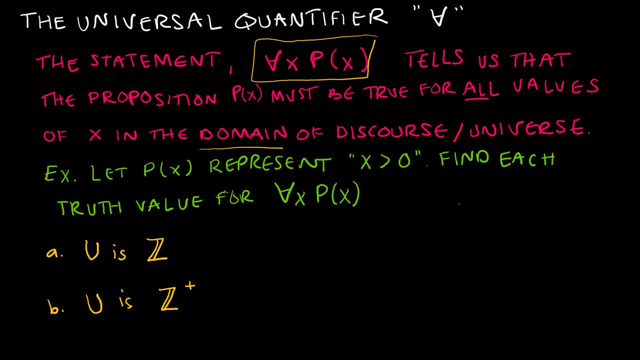 So domain, domain of discourse, universe, universe of discourse- these are all terms that you might see in your studies dealing with quantifiers. So let's take a look at an example. What we're saying is, if we have for all x, p of x, then in order for us to have a truth, value of true. 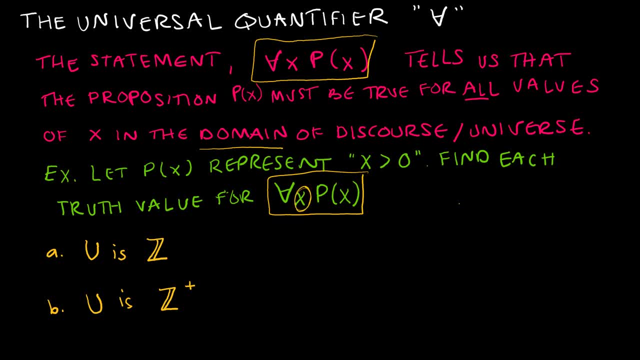 it must be true for every value of x in the domain. Looking at my first example, I'm saying: let the domain be z, which is of course integers. Integers are positive and negative, natural numbers and, of course, zero. So if it's all integers, to prove this is false, all I have to do. 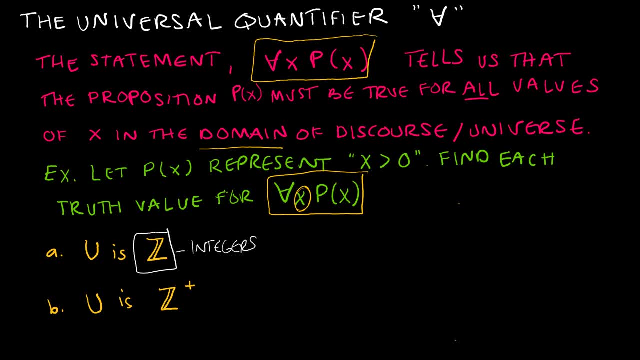 is find a counterexample. So let's use negative three. Negative three is in fact an integer and negative three is true. X greater than zero is false and therefore, for all x, p of x is false because I have found a counterexample. So in order to show something is false, all we have to do is find a counterexample. 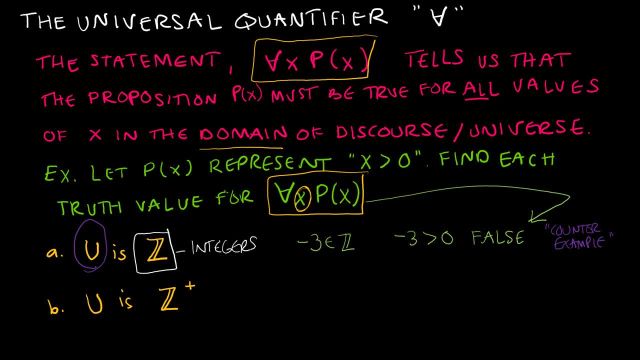 which is a value that is in the universe or domain, but shows us that the state of the statement, the proposition, is false. Now let's take a look at the next one. I have, now that the universe is positive, integers which would start with one and two, and three and four. 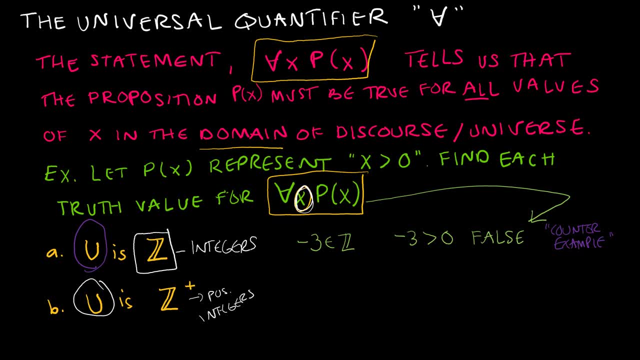 and so if I'm looking at all of those values, is it true that all of those values are greater than zero? Yes, So this is true. Now, that's not a proof, it's just our way of reasoning through it. So I didn't prove this. I showed by a counterexample, but I can't really do. 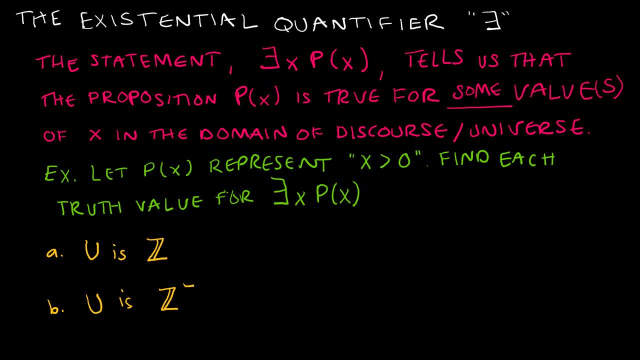 a proof for this. yet Let's now look at the existential quantifier Again. the statement there exists some x such that p of x tells that that the proposition p of x must be true for some value or values of x. Let's put some x here, I'll put some x here and I'll put 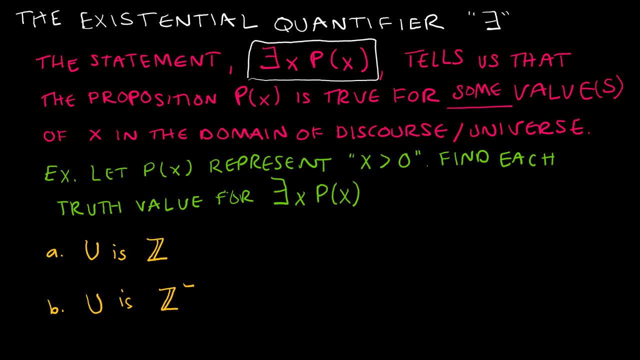 some y here, I'll put some y here, and I'll put some y here. Let's put some y here. Let's values of x in the domain of discourse. So how are we going to show? it's true? How are we going? 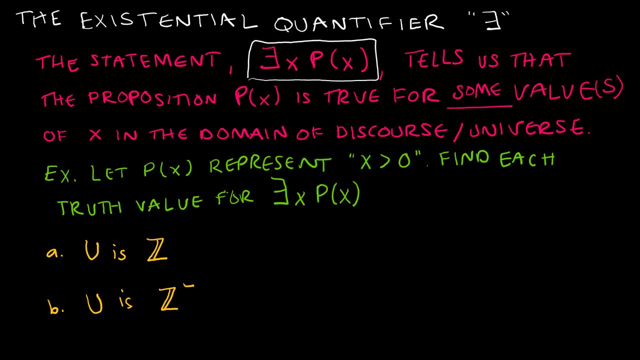 to show it's false Again. let's take a look at an example and hopefully it will make sense to us For u the universe of integers. using x is greater than zero. Can I find some integer that is greater than zero? Well, let's use seven. Seven is an integer. 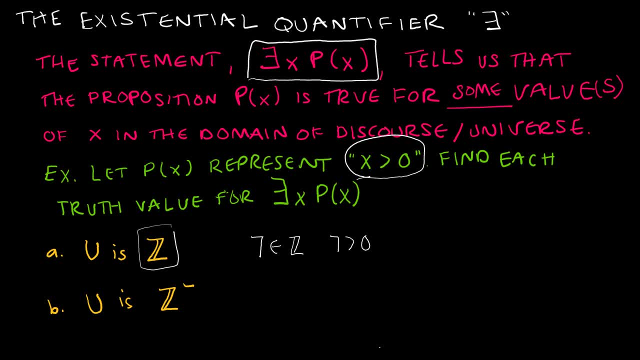 Seven is greater than zero is true, and all I need in the existential is to find one value that makes it true, because it has to be one or more. So, because I have found a value, it is true. Let's take a look at the negative integers: Negative 1, negative 2,, negative 3, etc. Can I? 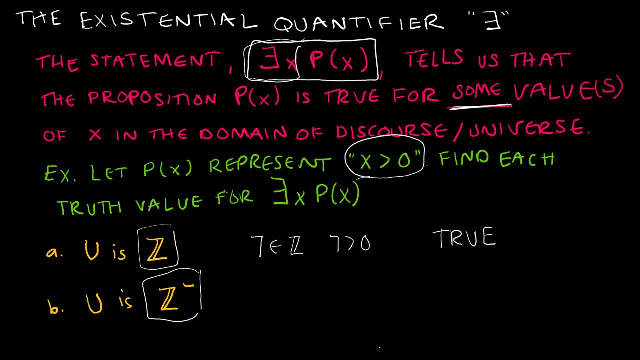 find any one of those values that is greater than zero. Well, all of those values are in fact, less than zero because they are negative and therefore that is false. Again, it's okay to just show an example. Let's take a look at the negative integers: Negative 1,, negative 2,, negative 3, etc. Can I? 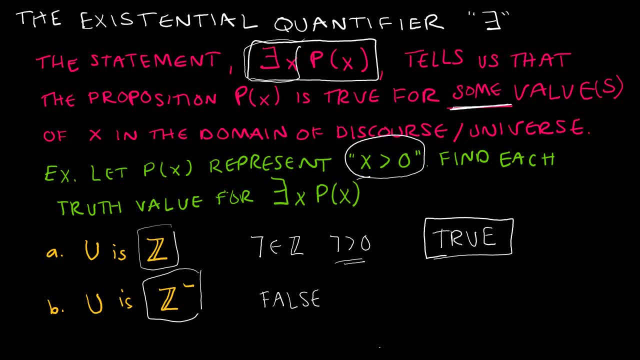 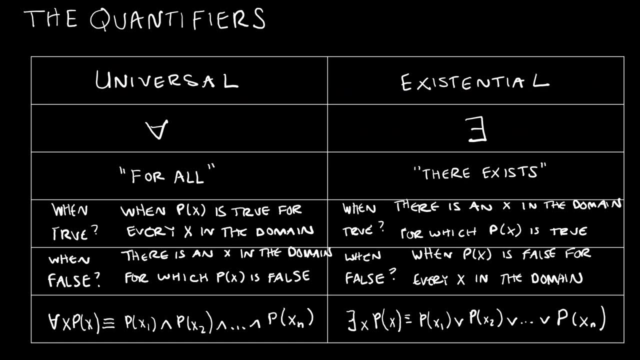 find any one of those values that is greater than zero. Well, all of those values are in fact, less than zero. Again, it's okay to just show an example, for true in this case, but for false it would require a proof, and we're not to that point yet. I wanted to throw this in here. This is just sort of an 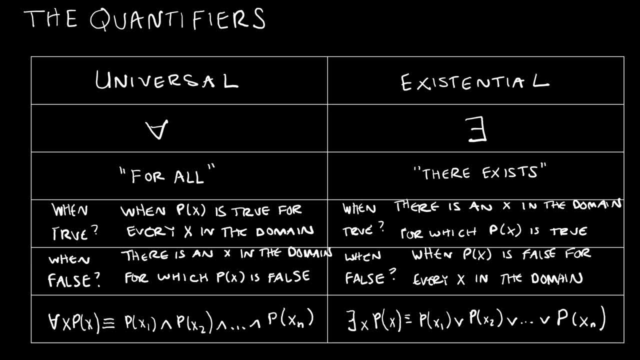 organizational system to make sure we understand the difference between the two. So we have the universal quantifier. on the left It's the upside down. A is the symbol. It means for all. When is it true? When p of x is true for every x in the domain. 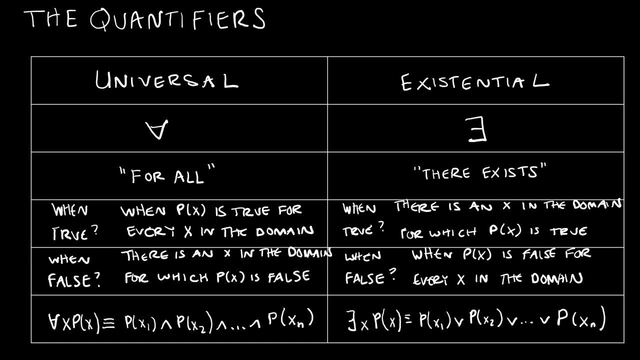 But it's false if there is just one x in the domain for which it's false. And then, of course, because we've been dealing with our connectives, the statement for all x, p of x, is equivalent to saying that it's true for the first x and it's. 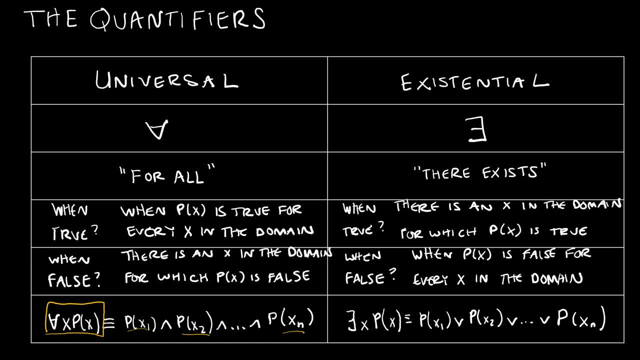 true for the next x, and it's true for the next x, etc. for every single value in the domain, Whereas the existential is the backwards e and means there exists. When is it true? When there is an x in the domain, for which p of x is true, So just there just has to be one. When is it false? When 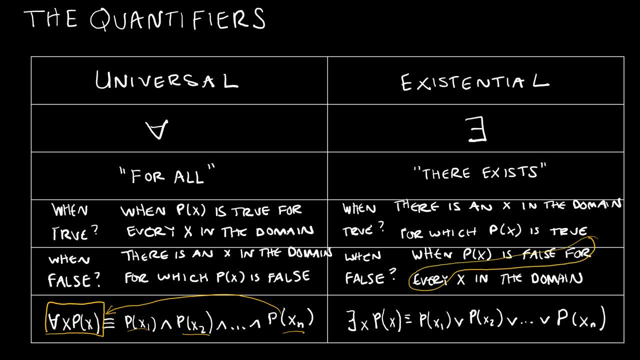 p of x is false for every x. So I want you to see here that these are sort of crisscrossed here For every x over here, for every x over here, whereas when it's true, when it's false is now, when there's. 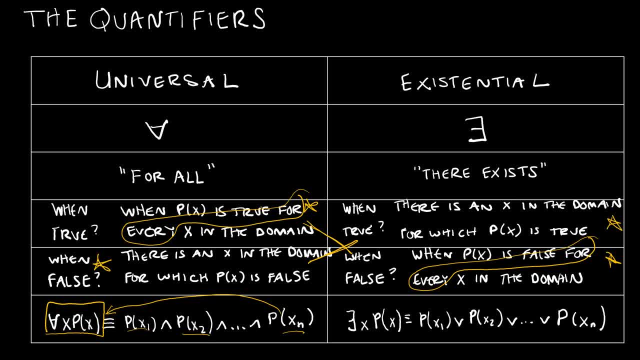 just one, when there is just one, And then of course there exists some x, such that p of x is true, would be, it's true for the first value, or the second value, or the third, And it just has to be true for one of those, And that's what that or means, Whereas and means it must be true for all. 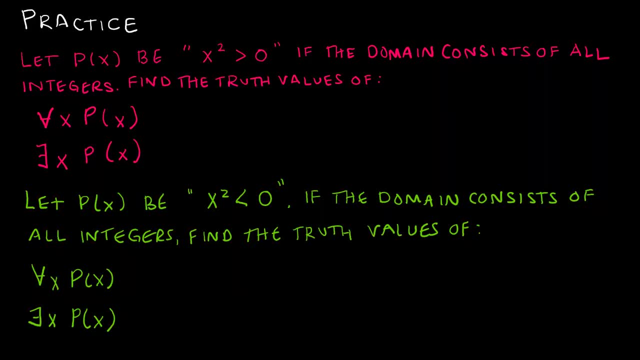 Here are a couple of practice for us to try, just to make sure we understand each of those quantifiers. So let p of x be, x squared is greater than zero, And the domain in the first example I'm looking at, the pink example, consists of all integers. So now I need to find the truth values. 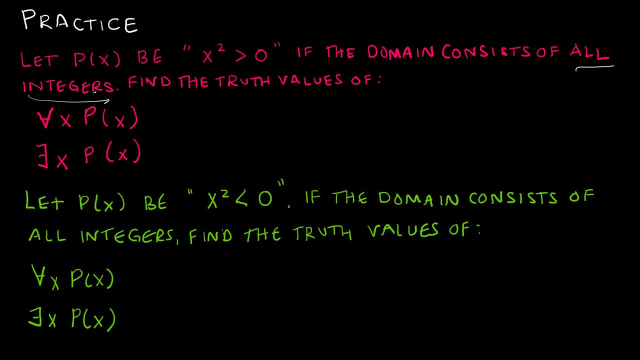 of for all x, p of x and there exists some x p of x, So x squared is greater than zero. So I'm going to find the truth values of for all x, p of x, and there exists some x p of x, So x squared is greater than zero for the value of 0.. 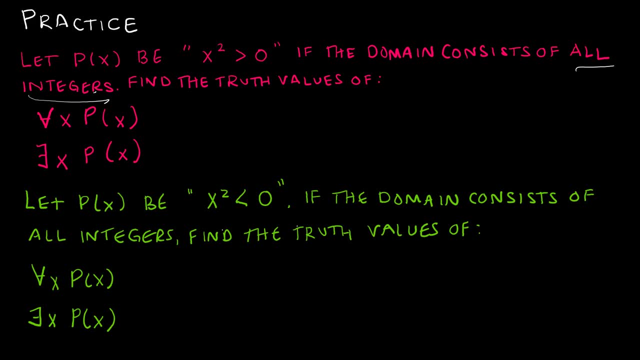 of all integers. Is it true that all integers, if I square them, are greater than zero? Well, almost. However, zero is considered an integer and zero, squared, is greater than zero is a false statement, And because I have found one counterexample, then this entire statement I'm going to put, therefore, for 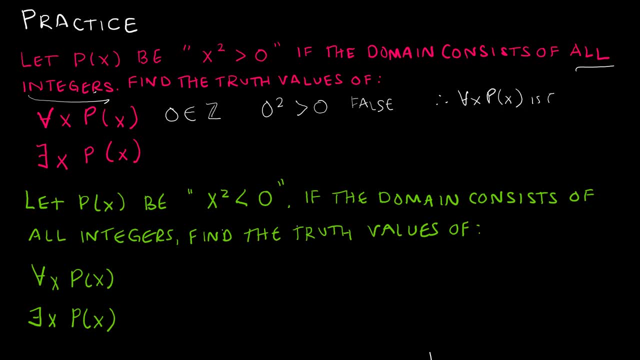 all X. P of X is false. There exists some X such that P of X is true. Well, can I find one integer like one? One squared is greater than zero. Sure, that's true. So all I have to do is find one. 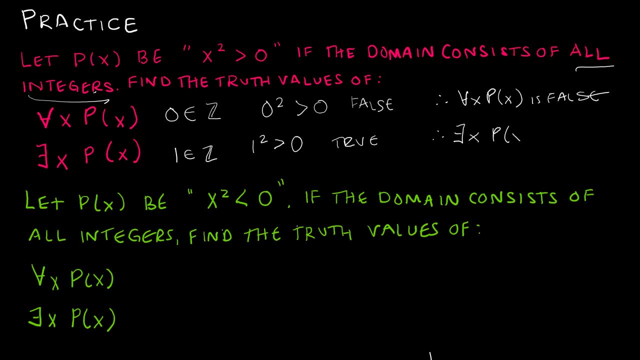 Therefore there exists some X, such that P of X is true is true. All right, now let's take a look at X. squared is less than zero For all X, P of X, so for every single integer, is it true that if I square it it's less than zero? 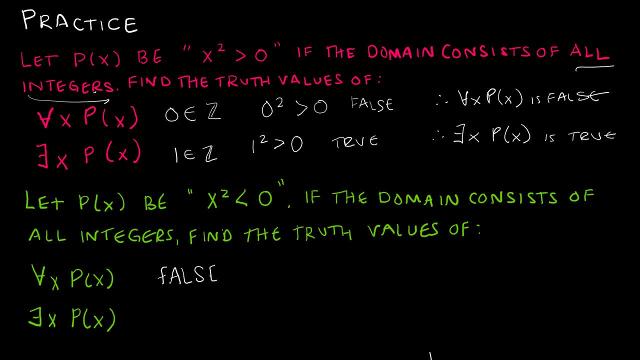 Hopefully that's pretty clear that this is false, Because obviously if I take negative one and square it, I get one is less than zero and that's false, And so if I find a counterexample, then the whole statement is false. So therefore, for all X, P of X is false. There exists some X such that P of X is true is true. Well, can I find one integer like one? There exists some X such that P of X is true is true. So therefore, for all X, P of X is false. 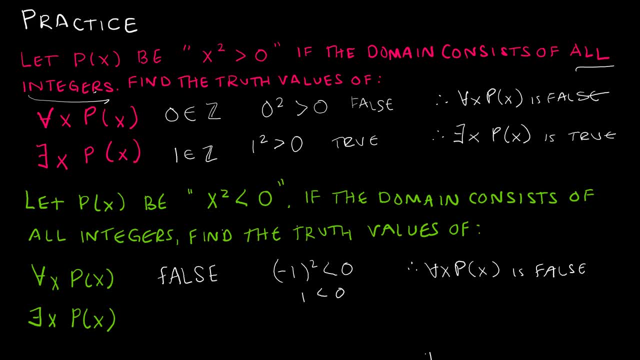 exists some x such that p of x is true. so is it possible for me to come up with some x that when i square it it is less than zero in the domain of the integers, and again, hopefully we know that that in fact would be false. now, one way you can go about doing this, and for most of us we can just: 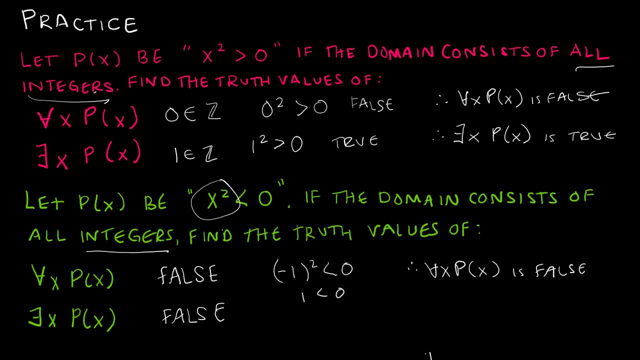 look at it and say, okay, well, there's no way to square something and get a negative value if we're dealing with integers, but you can always think about cycling through the value. so i can think about taking negative three and squaring it and finding out what happens. and negative two and 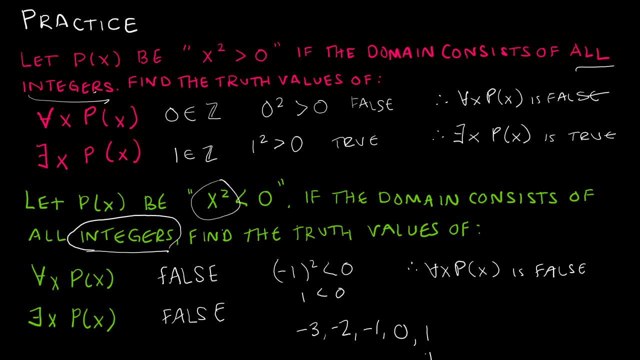 squaring it and negative one and squaring it and zero and squaring it and one, and two, and three, and i can go as far as i need to in each direction to test that, to determine the truth value. here are two more that i would like for you to try on your own. 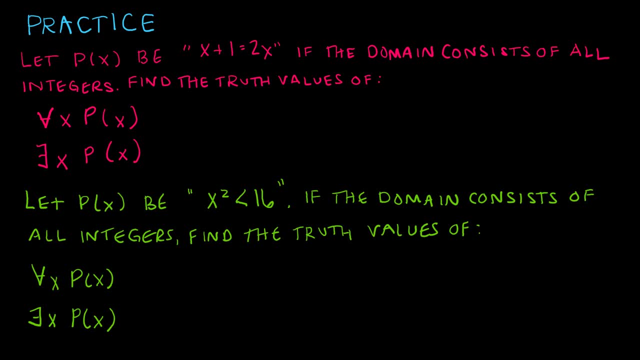 so if you would press pause, try all the parts of each question and when you are ready, press play to see how you did for the first one. we have let p of x be x plus 1 equals 2x. so what i would do is i would say x plus 1 equals 2x by subtracting x from each side, gives me x equals 1. 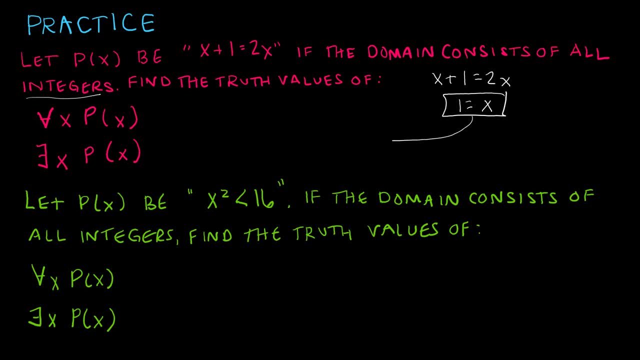 so to me again, dealing with the integers tells me, yes, there does exist, and there is an x. that means that x equals 1. so, yes, this is true. so i'm going to go ahead and think about this a little bit and we're going to go ahead and go ahead and see if there's any other. 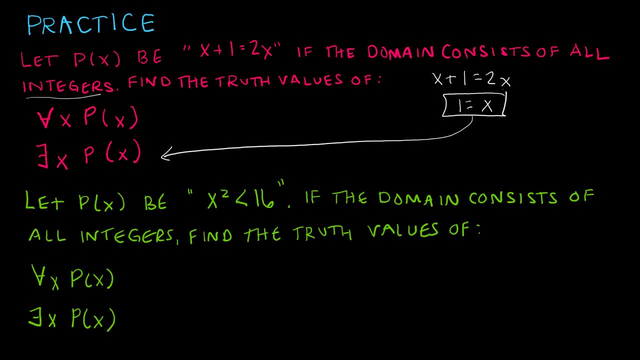 X, such that P of X is true, because I just found that the X is 1. so this guy is true. is it true for all integers? no, of course it's not. I can't plug in any old integer and find: have it be equal to 1. I can only plug in 1 and have it be. 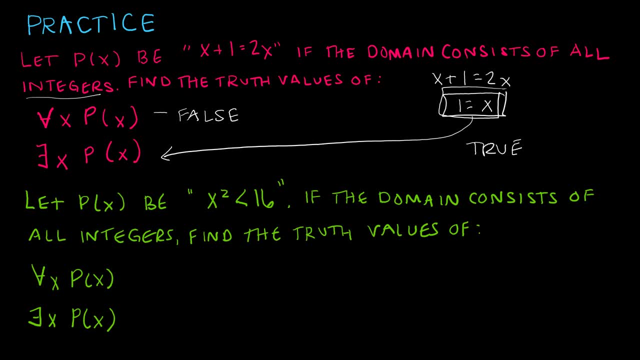 equal to 1. my next one, x squared, is less than 16. again, if I were to solve this, I would have negative 4 is less than X is less than 4 in order for that to be true. so does there exist some integer that is between negative 4 and 4? yes, so that's. 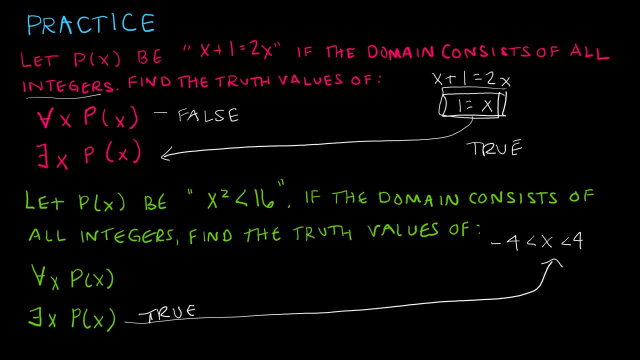 true, like 3: 3 squared is 9. 9 is less than 16 is true. so I have found an example that shows that it's true for all X's. if X, I'm sorry, if the domain is all integers, no, because I can find a counterexample. let's say 5 squared, oops, not greater. 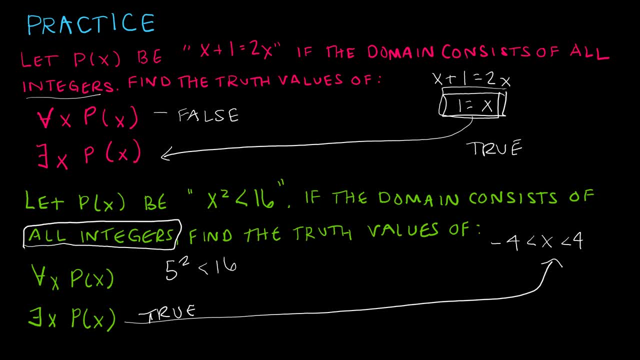 than 5 squared is less than 16, which is, of course. 25 is less than 16, which is false. so this is false. again with a counterexample, and I'm going to do the same thing for the other one. I'm going to do the same. 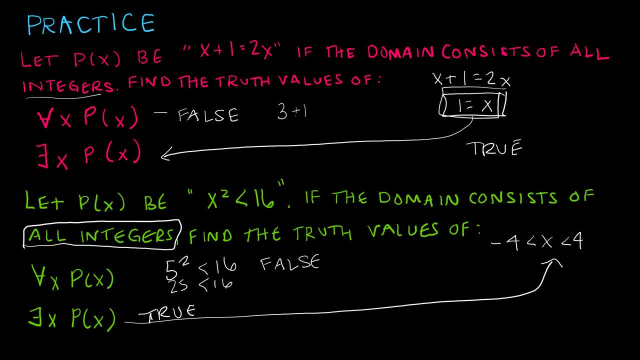 thing for the other one. I'm going to do the same thing for the other one. I'm going to use an exclamation point and I didn't have a counterexample up here, But I could have: 3 plus 1 equals 2 times 3, 4 equals 6 is obviously false. so 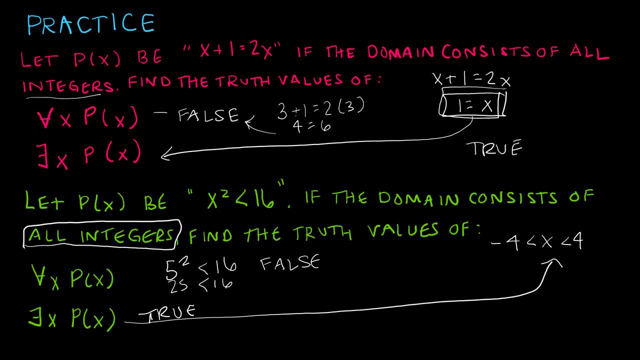 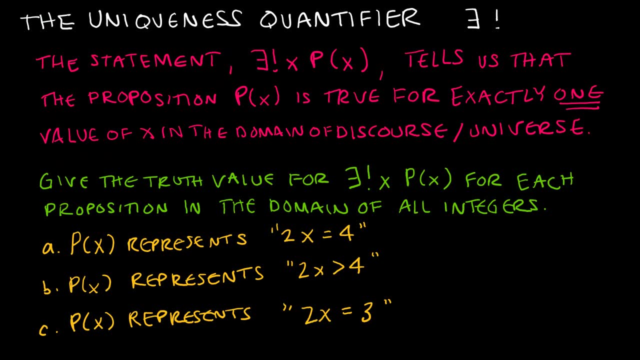 it's always good to give a counterexample. when you're saying false and true, we're just going to reason through it or explain why I did want to throw in one more quantifier, just because it's similar to one that we've already learned about: the existential quantifier. if you see that with an 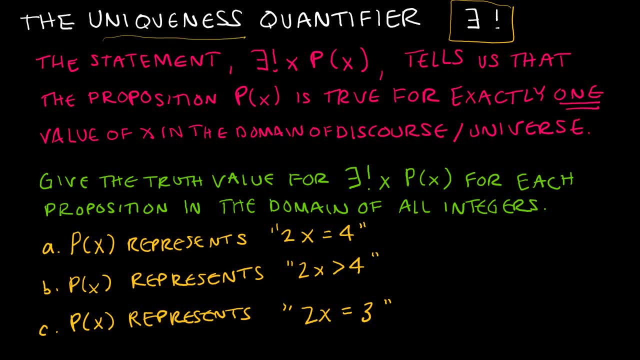 exclamation point. it's called the uniqueness quantifier and instead of saying there exists, it's essentially saying there exists exactly one, which means there exists a solution and it is unique, which is why it's called the uniqueness quantifier. so give the truth value, for there exists a unique X, such that P of X is true for each of these. 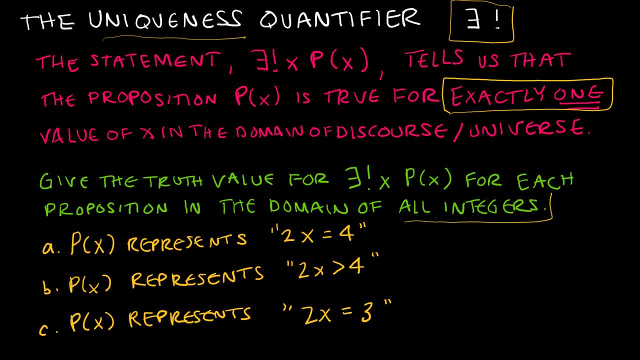 propositions and the domain is all integers. so, looking at the first, we have: P of X represents 2x equals 4. well, again, using oops, I was going to switch up my colors here. using basic algebra, 2x equals 4 is equivalent to X equals 2.